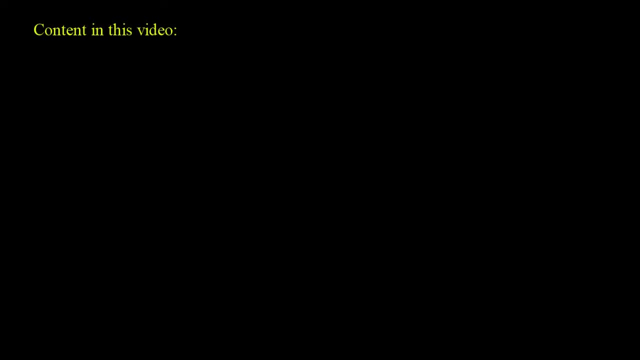 So today I'm going to teach you how to graph the most common trigonometric functions, sine and cosine, without using a calculator. You actually only need to know the transformation factors, which are the amplitude, the period, the phase shift and the vertical shift. 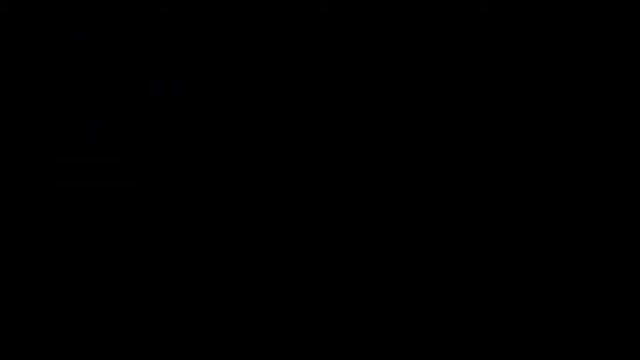 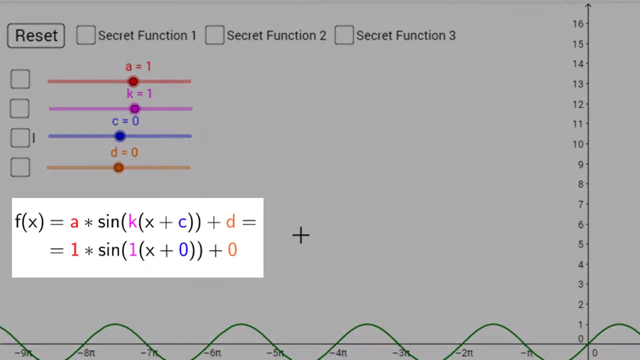 for a trig function to be able to graph it, And we can determine all these factors from a function's expression. And this video will also include some examples where you can test your new knowledge. So let's get started. So this program is showing a graph of this sine function over here, which is written in a general 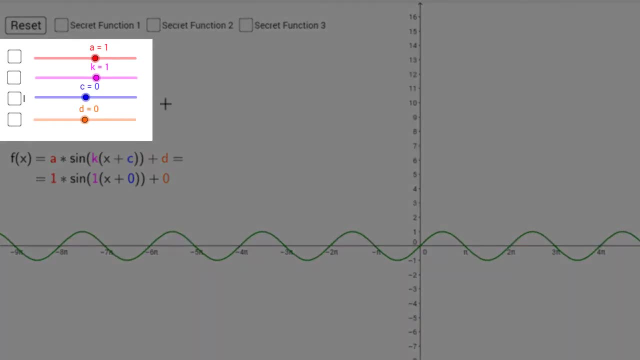 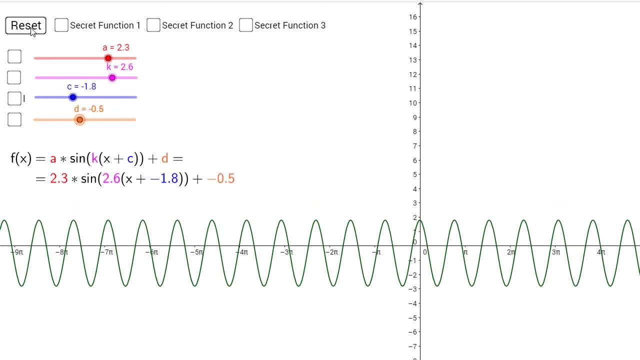 form And the sliders here at the top let me change the variables in the function. And of course we also have a reset button that let me reset all the sliders. But now we're going to try to make some connections between the transformation factors. 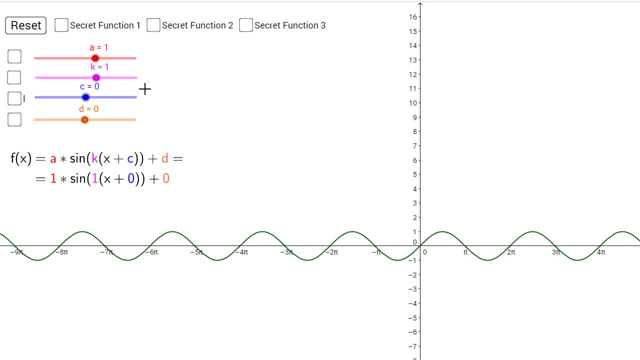 and the variables in this function. Let's start by trying to change the a value a bit. So by increasing the value of a, we can see that the amplitude of a function, which is the distance from one peak to the center line, seems to increase. And that's also the case. 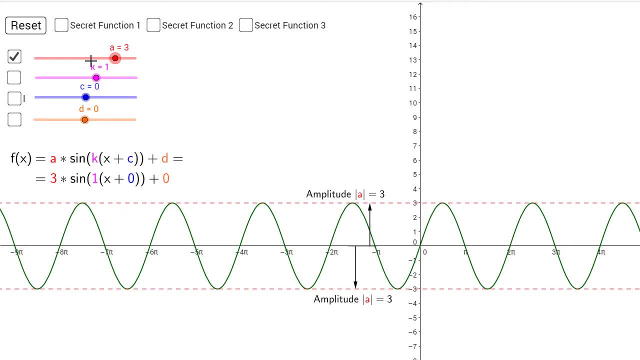 because the amplitude for a trigonometric function is equal to the absolute value of this variable a. The next variable is k And we can see here that the period, which is the distance between two identical points, shortens with bigger values on k And the connection between the period and the k. 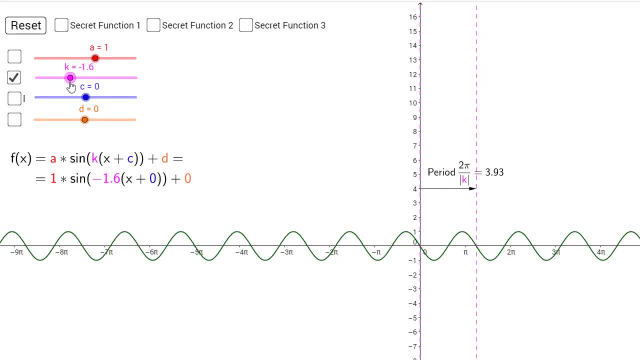 value is that the period is equal to two pi divided by the absolute value of k. So okay, let's skip c for the time being and move on to d. The variable d is in charge of the vertical shift of the function. So if you increase d, you will see that the function is raised a bit. 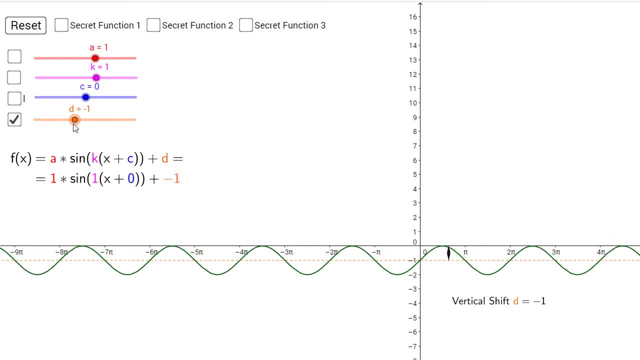 And if we decrease it we can see that it lowers the whole function. So now we only have a phase shift left and only one variable left, And the connection between them is that if we increase the variable c, we'll see that the function is moved to the left. 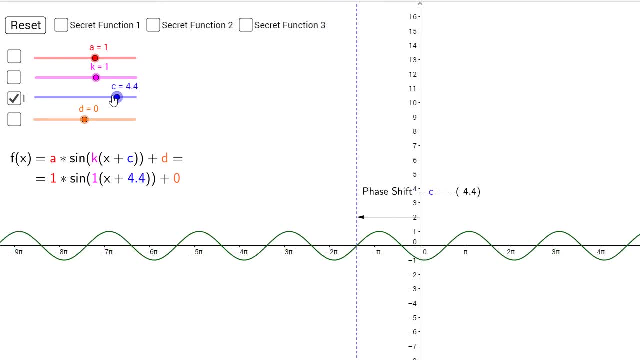 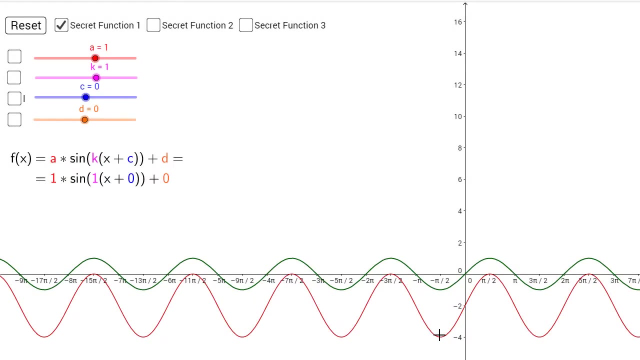 And if we decrease it, we can see that the function moves to the right. So the phase shift for a trigonometric function is equal to minus c. So, with that said, let's move on to some examples. I will add a secret function, this red. 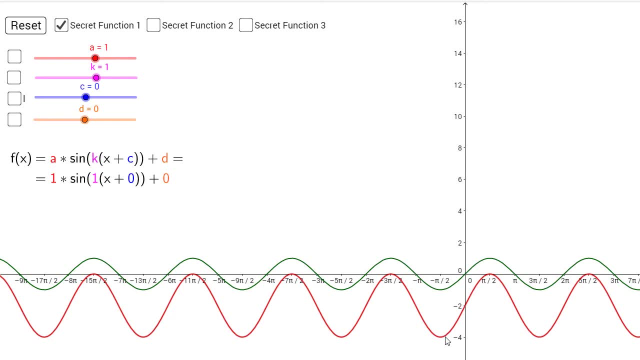 function here. I would like you to pause the video and try to determine the transformation factors for this function. Let's start by determining the amplitude, and the amplitude is the distance between one of the peaks, the highest of the lowest, and the center line. 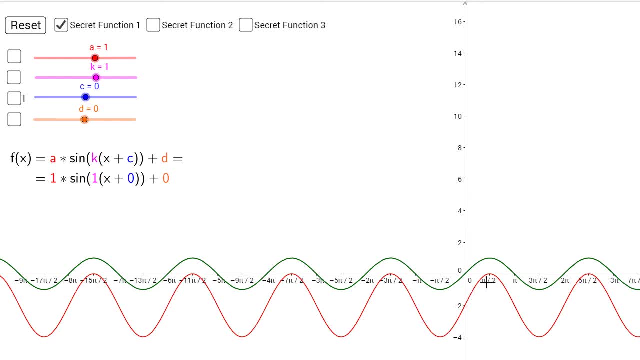 which in this case is minus two, and we can see here that the highest peak is zero and the distance between zero and minus two is two, and therefore the amplitude is going to be two. Let me plug that in right away. Yeah, that seems to match pretty well. 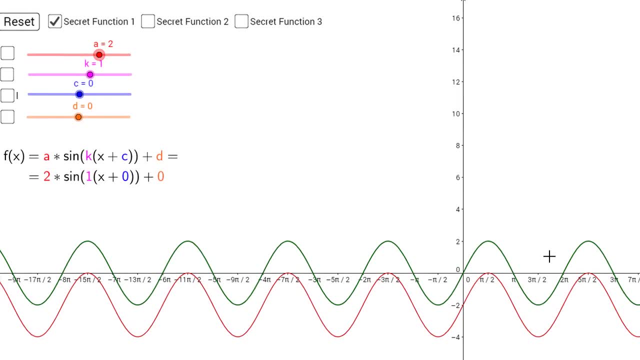 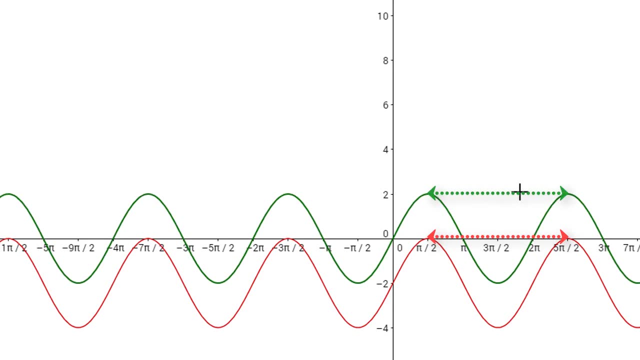 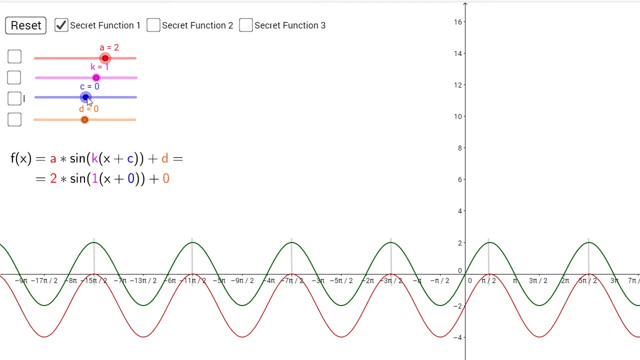 Let's continue with another transformation factor. We can observe in the graph that the peaks are on the same distance from each other for both functions and that means that the two functions have the same period, and we can also see that the peaks line up. 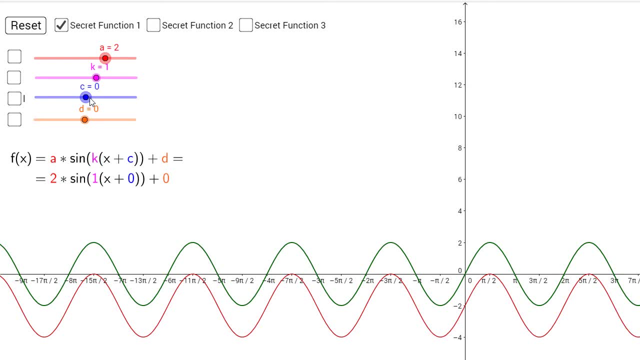 so there's no phase difference between the two functions either, but the red function seems to have been moved two steps down, so therefore the D value is going to be minus two. So that was one example to determine a function's transformation factors by just looking at the graph. 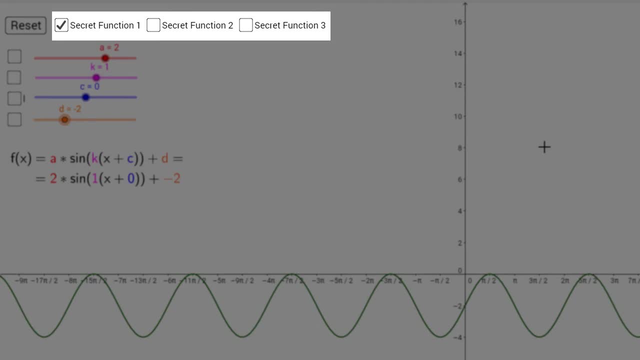 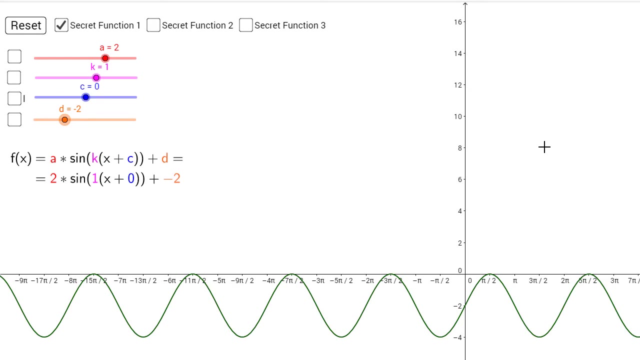 But actually we got two more secret functions but at the same time. I don't want to bore you, so I will just link this program that is free to use in the description so you can play around with it yourself, and please let me know in the comments if you've tried it. 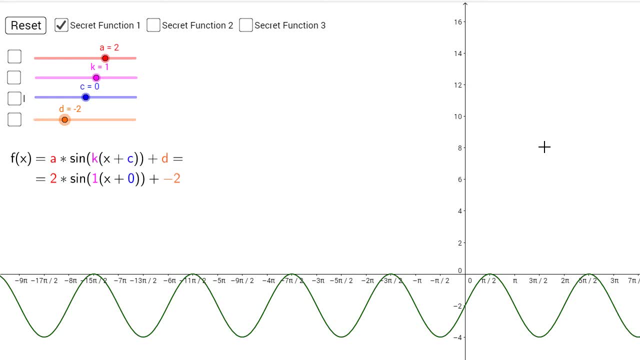 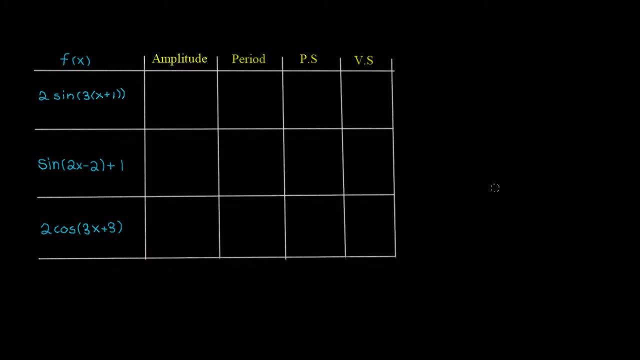 and I'll see you in the next video. Thanks for watching. I'll see you in the next video. Bye, Bye, That's a good thing to remember, So let's try to do the problems. Our first function is two sign, three times x plus one. 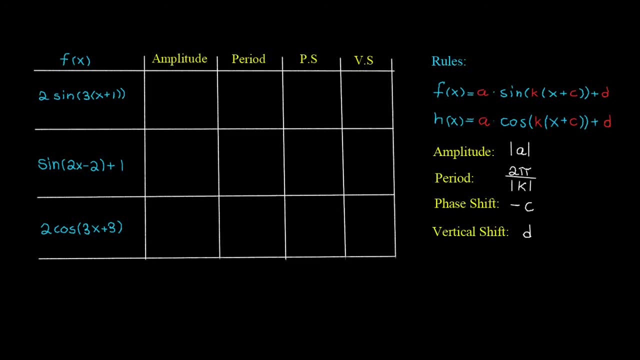 And if you use the rules, we can see that the amplitude is going to be two, since that is the number in front of the trigonometric function, and the period is going to be two pi divided by, divided by the absolute value of k. 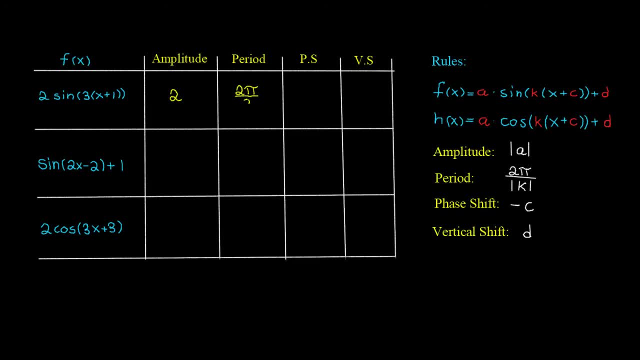 And k, in this case, is three. so the period is therefore going to be two pi divided by three. The phase shift is the same as the negative of the z value And since our z value was one, our phase shift is going to be minus one. 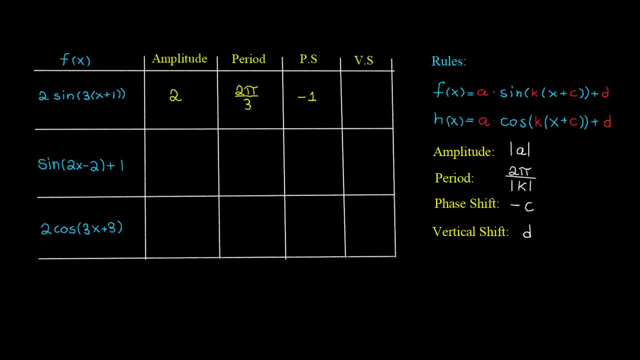 And we can also see that our d value is going to be zero, since our function don't have a second term to it, And our vertical shift is therefore also going to be equal to zero. The next function is a bit trickier, because we know how to handle trigonometric functions. 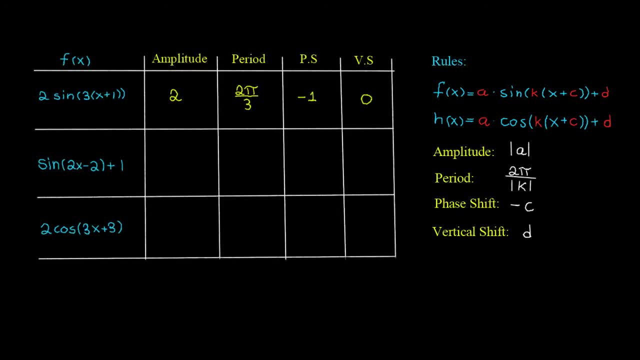 that are written in this form here. But this function here is not exactly the same, as you can see. We are missing the k value, but we can fix that. Let's try to rewrite our function so that it matches our formula. Let's see: sine two x minus two can be rewritten as: 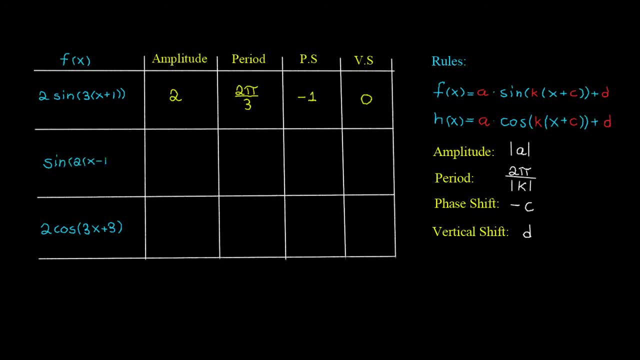 sine two and brackets x minus one. And now we have it written in the way we want, And now we can, quite easy again, with the help of rules, determine the different transformation factors. Let's see here: The amplitude is going to be one. 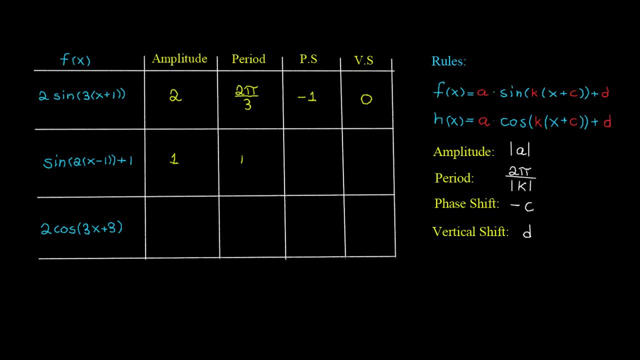 The period is going to be two pi divided by two, so pi And the phase shift is going to be: let's see, c is minus one, so the phase shift must be minus minus one, that is one, And the vertical shift is one here. 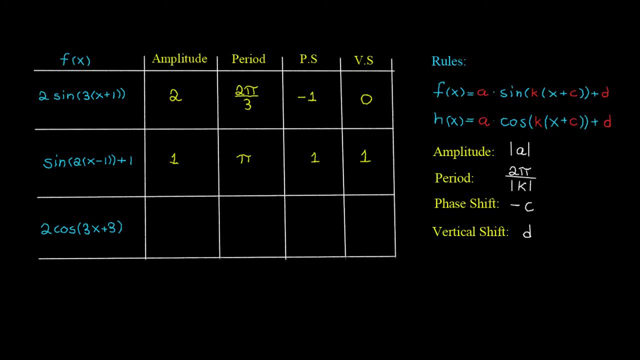 And for the last one, we need to remember that it's not only the sine function this rules apply to. it's also for the cosine functions. So, first off, we need to rewrite it as the one before And we get- let's see now- two cosine of three times.